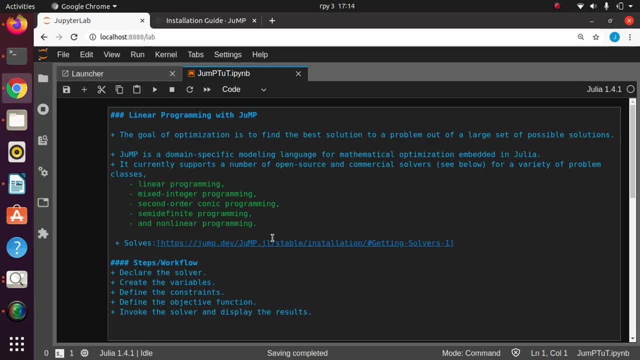 perfect, so let's see how to work with it. so in doing every format of optimization problem, a specific linear problem problem or programming, what you're supposed to do, you must first of all define or declare the server that you want to use. there are several servers, as you can see from here. 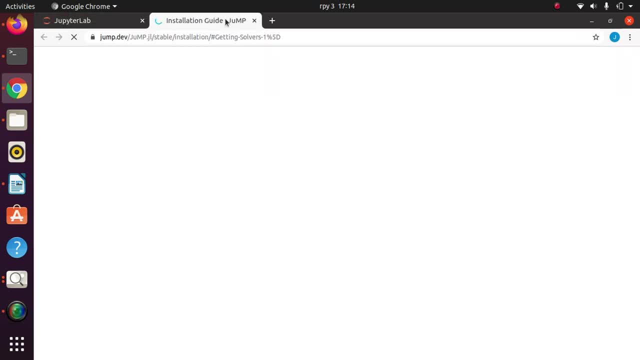 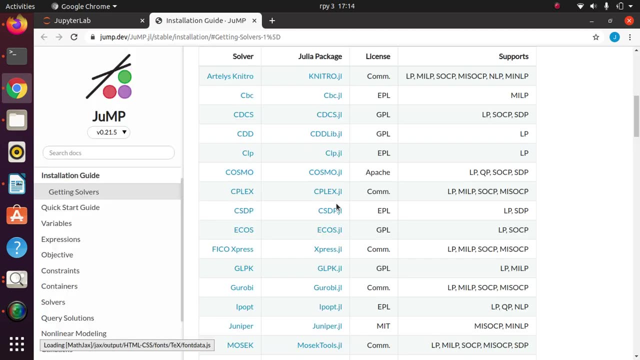 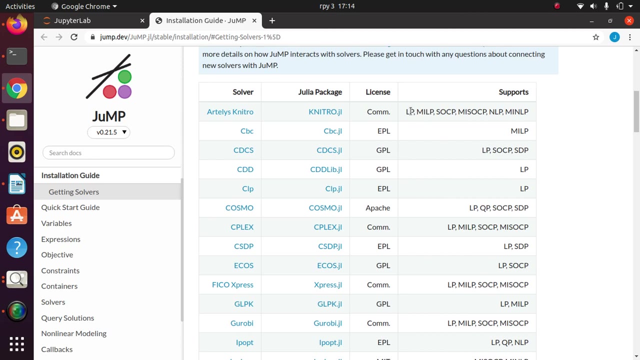 we have several servers i can use in julia, so most of these servers have support for different types of problems that you want to solve. so you can see from here that we have different servers. so these are the servers and then these are the particular support they have, so linear programming missed. 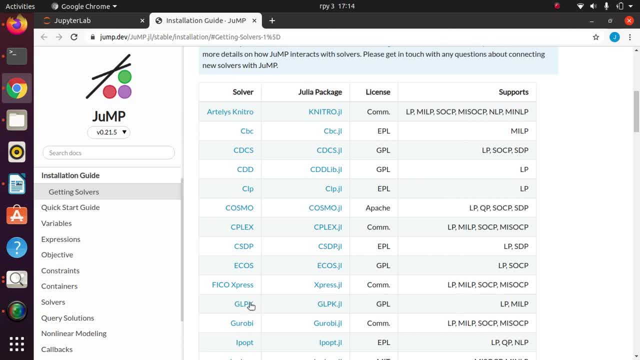 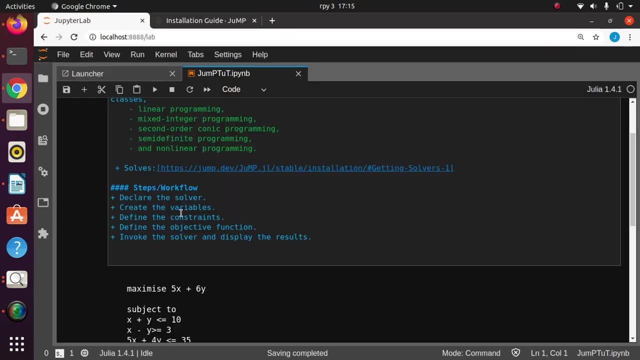 integer, linear programming and the rest right, but to be using this particular service here, so be installing it for this particular session. perfect, so that is the first thing. then you declare your variables, then you define your constraints or your limit. then you find objective function, then you invoke your server. so let's pick a particular problem and try and 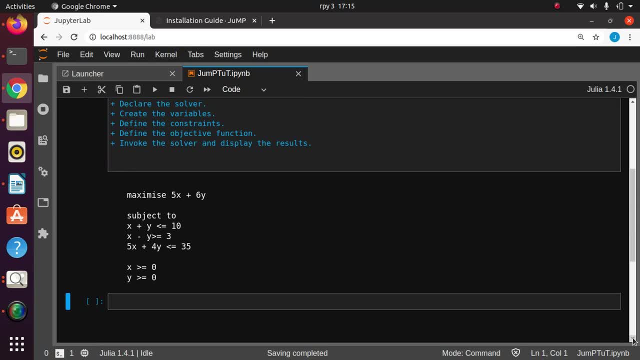 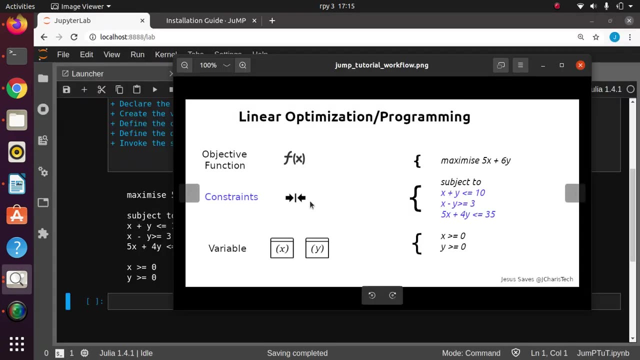 see how to use linear programming, using jump, to solve it. so this is the problem that you have: you are supposed to maximize fs plus this y which is subject to this particular constraint, and these are our variables. so a simple picture. is this a simple picture to help us understand that anytime you're giving something like this, 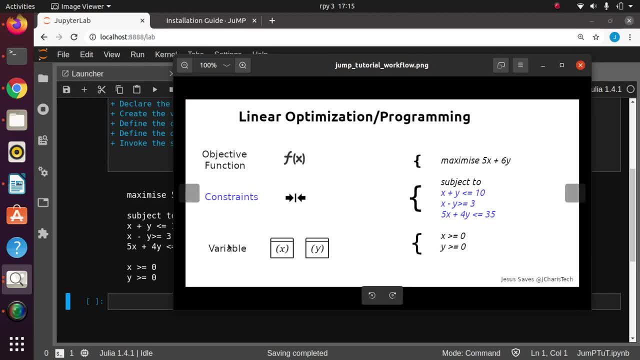 so we have three key elements. so you need your to know your variables. so these are going to be our variables as and why. right, in this case this x and y, which is going to have an upper or a lower bound. it might not be less than zero, right? perfect, then we also have our constraint. 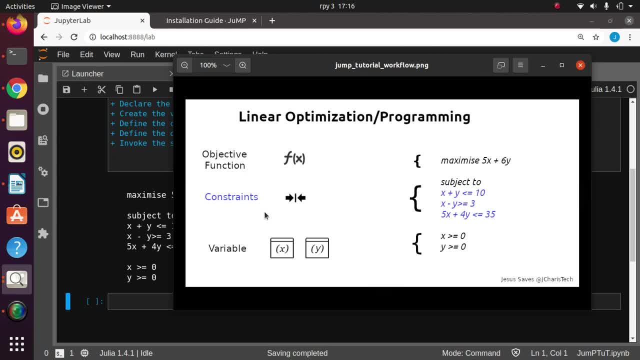 so the constraint is going to be the limit. what are our constraints, what are our restrictions for our activity, for the task we want to do? so this is, it's very simple. in case you are given a question like this: just what is stem subject to? so this is. 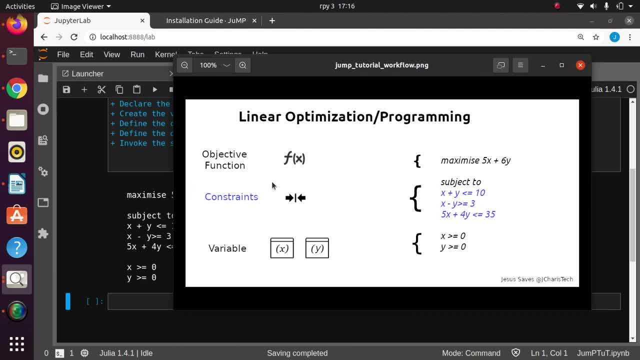 going to be our constraint? then the next thing is our objective function. what is our goal? what do you want to achieve? right? so our goal is to maximize this particular function, fx plus this y. so that is our objective function. so the three elements, your variable. you define your variables. 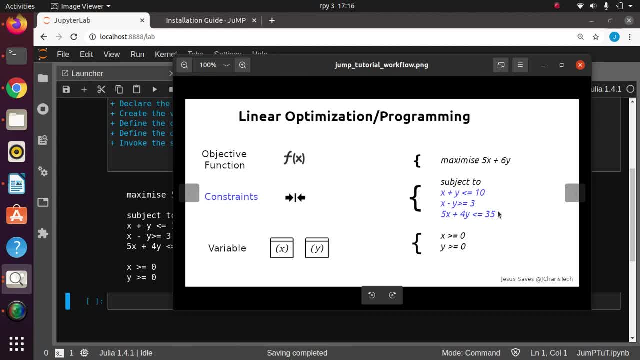 or you create your variables, you specify your constraint, it's very simple. then you specify the objective function, so it's going to maximize or minimize. so let's see how to work a little bit with it, so i'll just come back again to my chipta notebook. then you load, jump right so 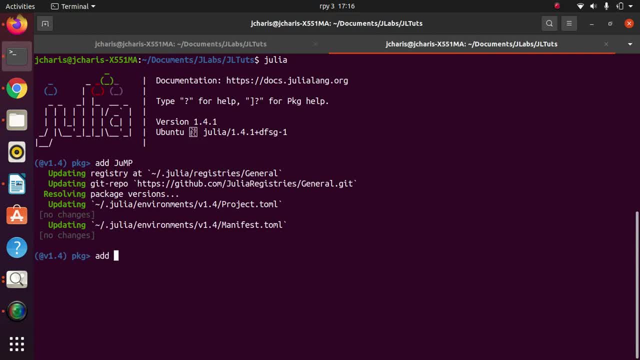 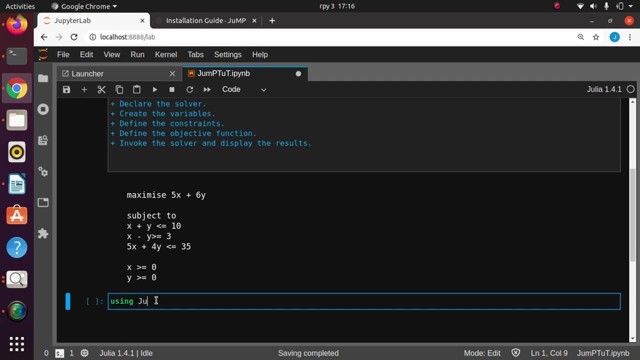 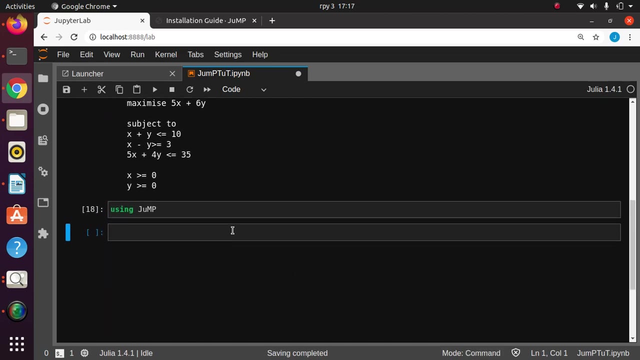 by now it has finished installing. so let's add our server. so add glpk. right, we're going to add our server. then i'll come back again and then we'll just load my package. so we jump to load our package, perfect, and then from here we will try and see the various methods of this. 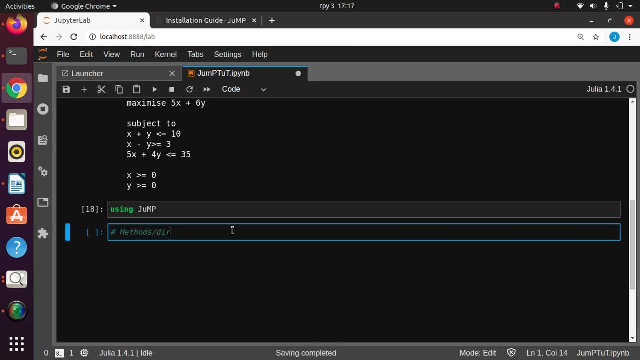 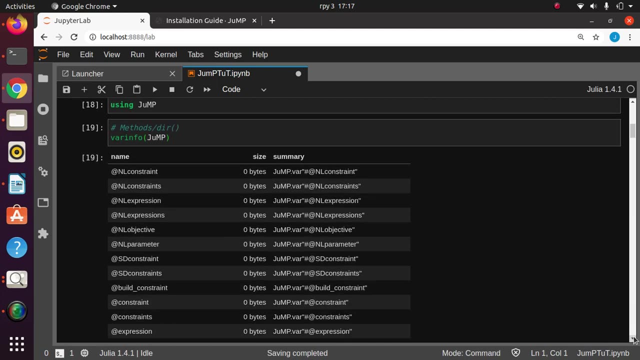 particular package- so they're going to be the methods- which is similar to drl- this option in my var info i'm passing my jump package right. so jump is going to give me all the various methods and activities i can do, and from here you see that we have several macros right. so the most 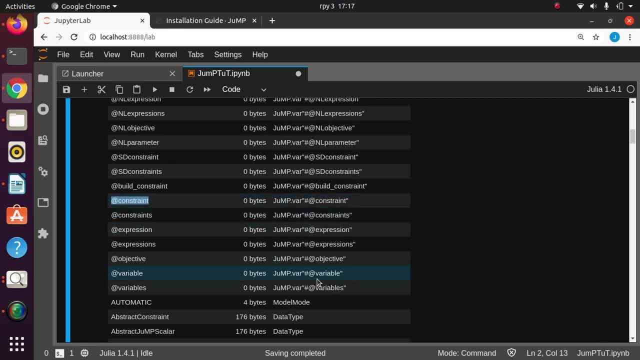 important one we're using is the constraint macro to define our constraint. we have our variable macro to define our variable. so we have four single and then for multiple pivot and also have our model, which is this right pivot. so let's see how to record it. so, first of all, we need to create 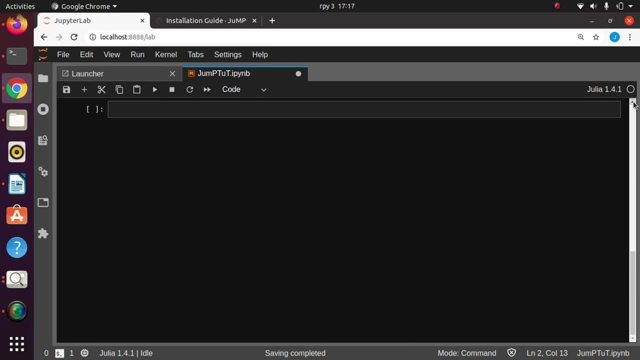 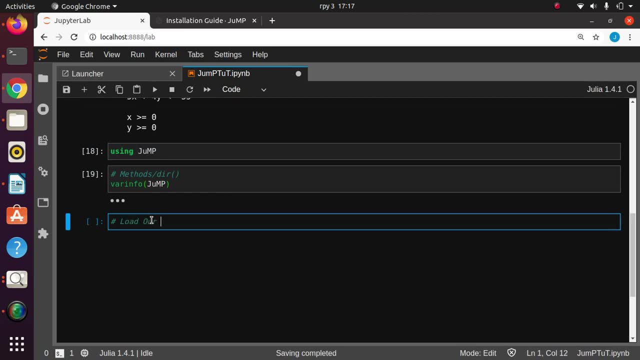 our model and then declare our solver right. so let's specify not to load our server. it's going to be my using jlpk. then from here i'm just going to. first of all, let's define our model. it's going to be m for model right, it can be anyhow. i'm going to call it as my model. 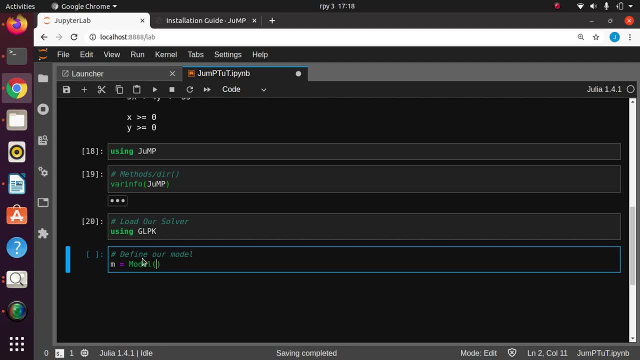 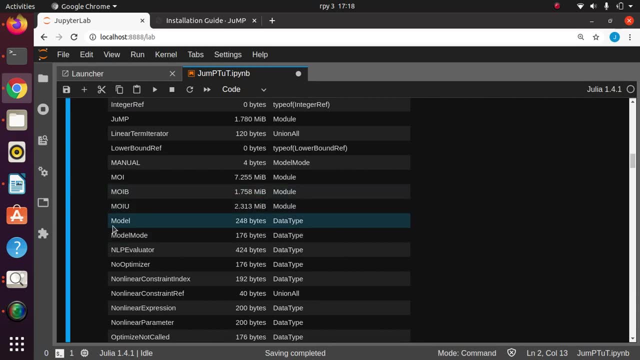 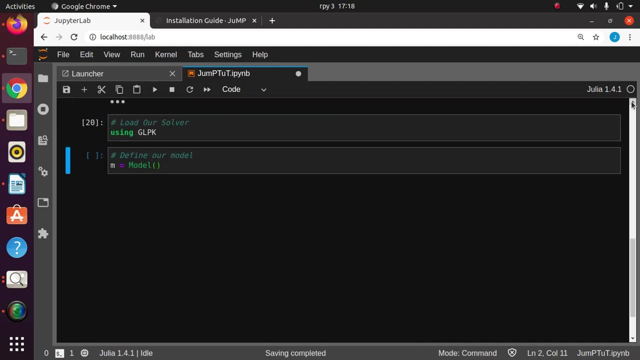 which is coming from jump, as we saw earlier on. so, model here is the model coming from jump, here this particular one. right, it's a function or data type, right pivot. then i need to specify the particular server. what do i want to use to solve my question? right, i'm passing my jlpk dot. 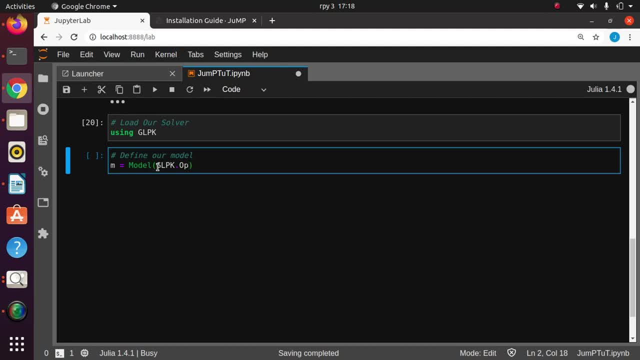 optimizer. so there are several ways you can do. so that is the simplest option, right? perfect. so now we're going to create our model, then we're going to specify the server we're going to use. perfect, now let's first of all create our variables. so, based on the question, 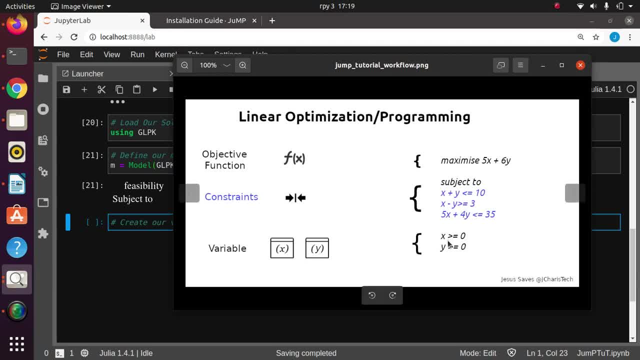 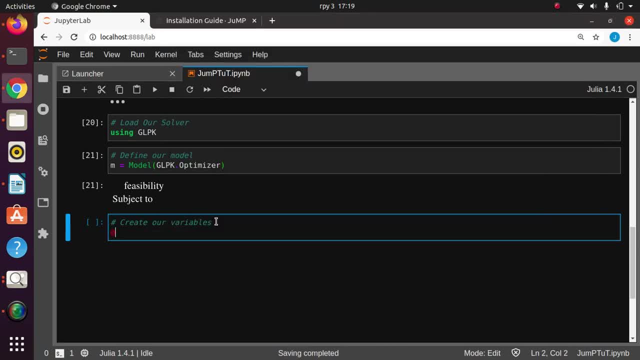 that we had, which was this particular question. so these are variables x and then y. right, so we're going to specify our variables, we're going to create a variable. so to create a variable, very simple, just go with the macro variable. then you specify the model, then you specify your variable. 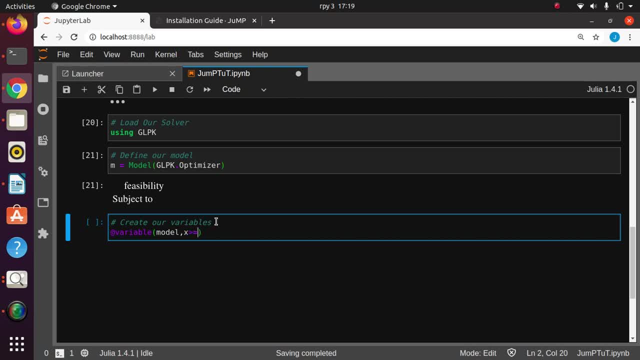 so x must be greater or equal to zero. right then let's create another one, so variable, for the model. this is m. let's go to m. we can just call it model anyhow you want it to be. so let's call it m for model. see, first time, so model, and then we just 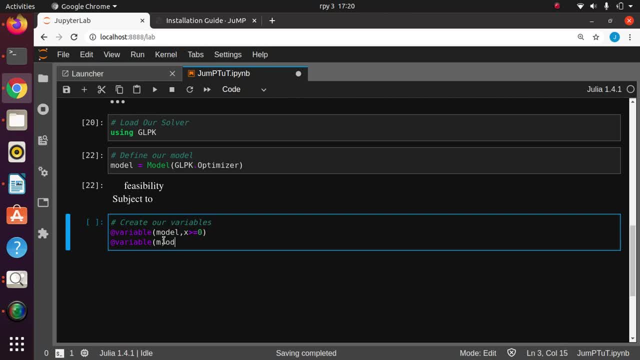 come back again so that it makes it easier for future people to remember. right, pivot, then this is going to be y, so these are upper, our lower limit. right, it might not be more than this pivot. we have critical variables. now let's say that this is going to be our model, so we're going to call it. 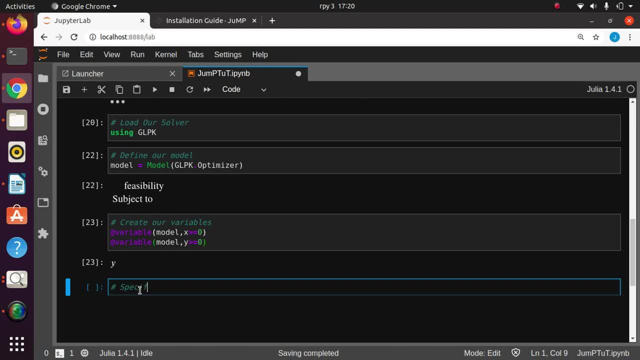 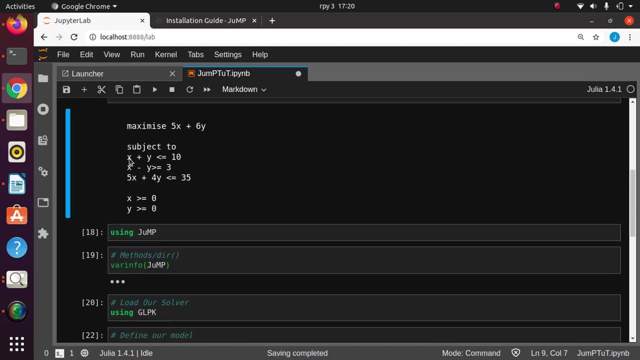 now let's specify our constraint. specify constraint. don't know how to spell constraint, and one thing is that anytime you are given a question like this question that we have here, something like this, it's very simple for you to know the constraints, right? so this is the constraint subject to the constraint. so let's try and see how to do that. 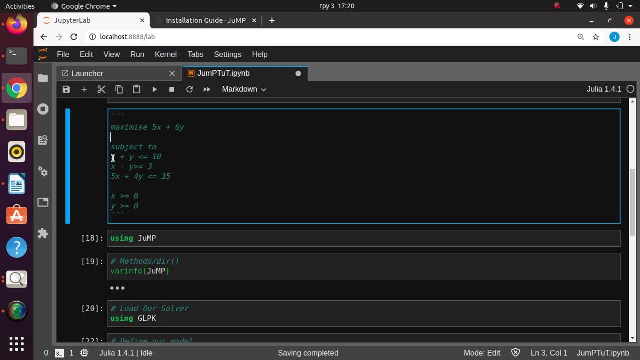 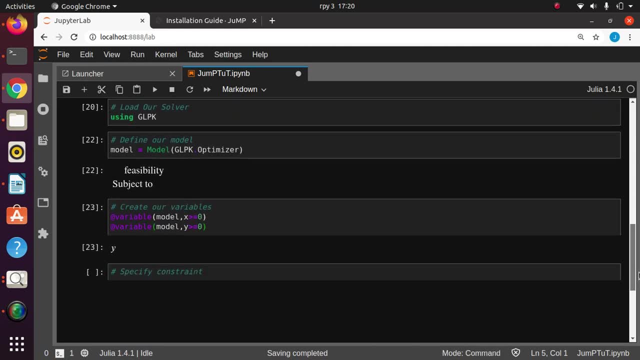 so this is the constraint and then this is going to be our variable. so we have defined our variable. let's work on our constraints. so i'll copy this one. i don't know that the audio is is behaving, but let me know in the comments section below. so to specify the constraints with the macro constraints: 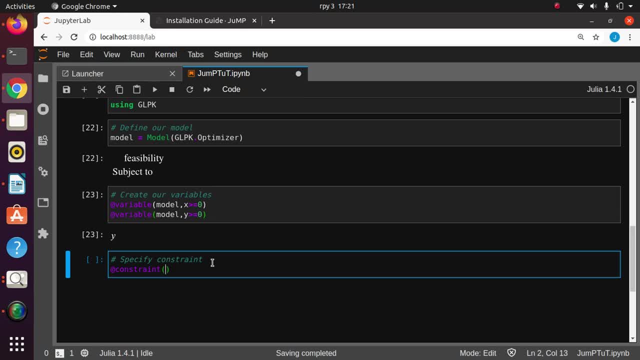 right constraint. then you just pass in your model as usual. then you specify the constraints. so this is going to be our constraint for the first one, so let's make it like this. and then this, the macro constraint, our model, and you specify right. so that is something very simple. 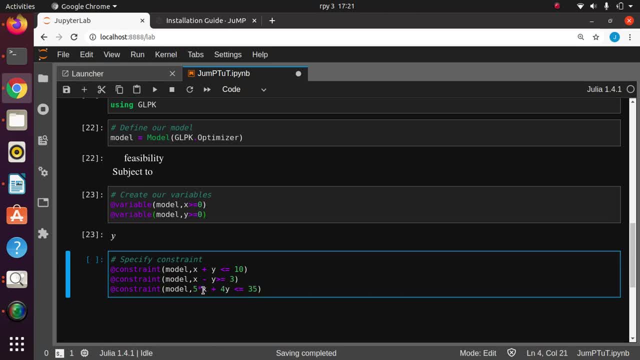 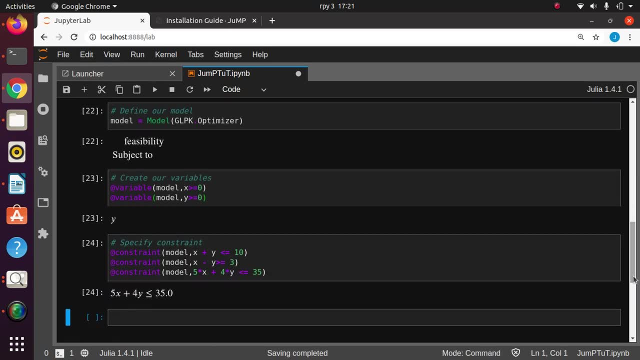 and once you have to notice that when you are doing this, you should make sure that you multiply this, right, because it works perfectly well. so this is going to be our constraint, perfect. so we have done. we have gotten our model, our variables, our constraint. now let's define. 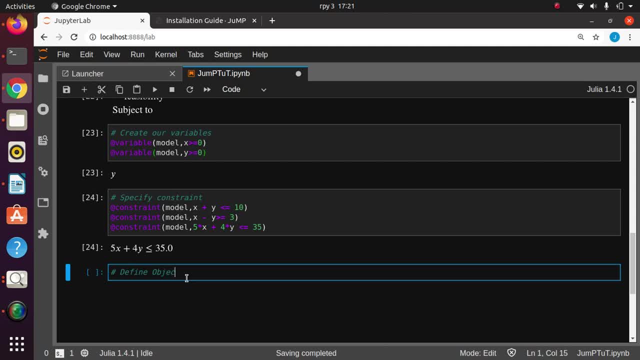 our objective function. so it's very simple, just go with, add the macro objective, right, it's going to be our objective function. then you specify your model. then you, what do you want to do? so this one takes three argument: the model, then in our question that we had, we are supposed to maximize something. so that's going to be the 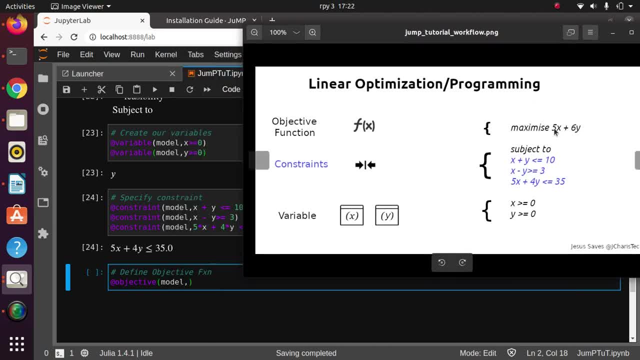 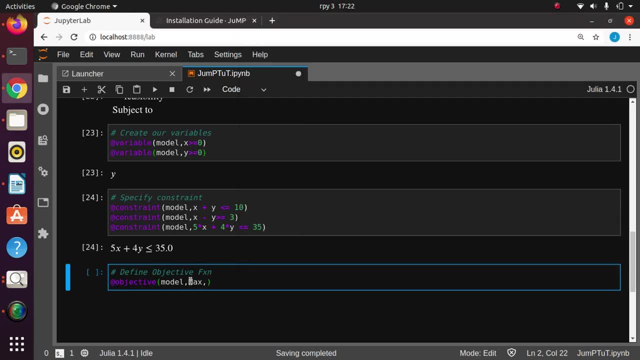 next argument: we're supposed to maximize something. then i'll paste in 5x plus 6y. very simple, so we're supposed to maximize. then what are we maximizing? 5x plus 6y. so in the next argument, we are supposed to maximize something. so that's going to be the next argument. we are supposed to maximize something, then i'll paste in 5x plus 6y. very simple, so we're supposed to maximize. then what are we maximizing? 5x plus 6y. 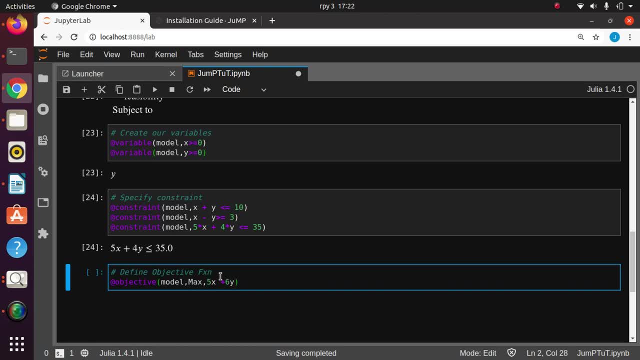 so in the next argument we are supposed to maximize something. then i'll paste in: 5x plus 6y, very simple. so we're supposed to maximize, then what are we maximizing? 5x plus 6y. so in this case, don't multiply, it just goes. 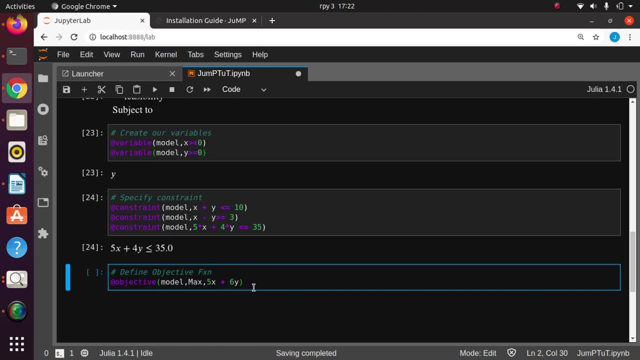 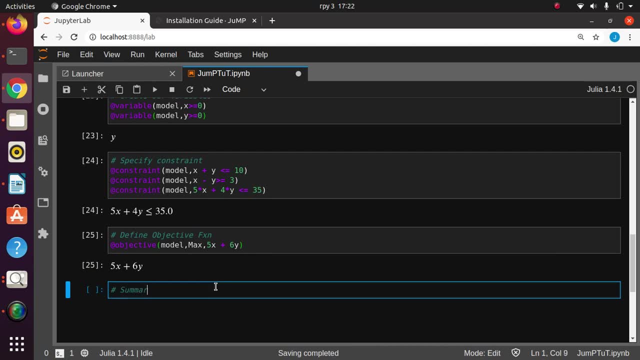 straight away with this, right, you don't do this, it's going to understand it. so that is our objective function. you have to find them now to see everything that we have done so far. a simple summary, very simple. just go with my macro. show: you can use display anyhow you want it to be, so show. 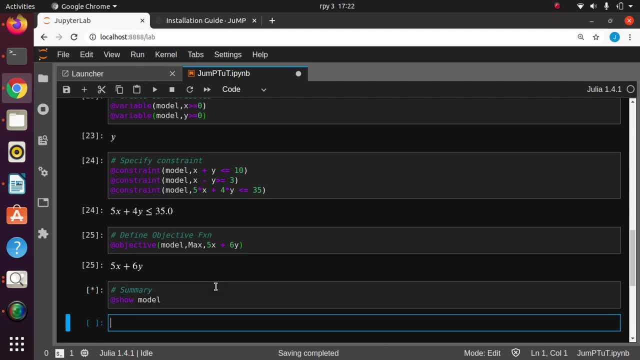 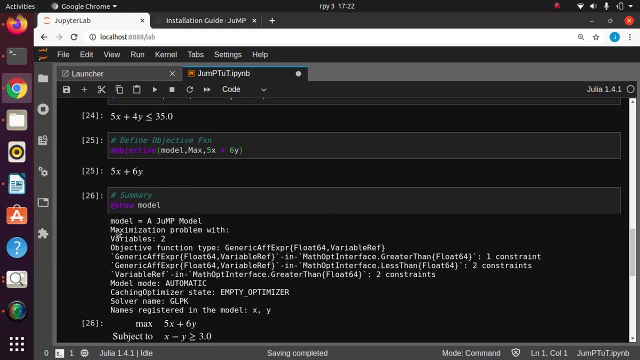 show then my model. so this will give us a summary of whatever you have done. so, based on the summary that we have our model, we are using a jump model and we are supposed to maximize. it's a maximization problem, as we specified here, and we have two variables, x and y, and these are: 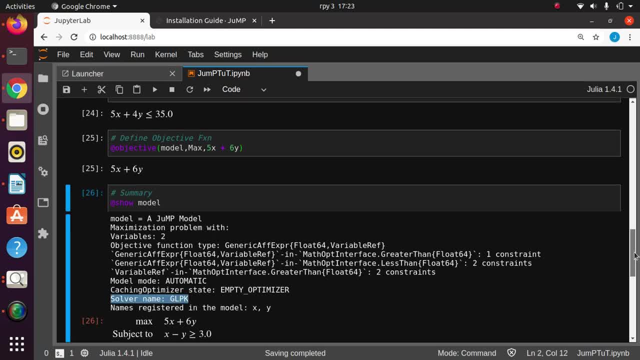 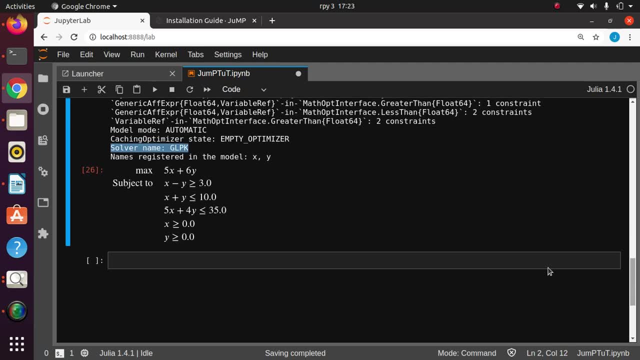 solver, and then this is exactly the same thing that we we saw in the question below. so you have to get something like this. that means that it's simple for you. you can solve it right. perfect, now let's see how to solve it. so to solve it is very simple: just give it solving or optimizing. 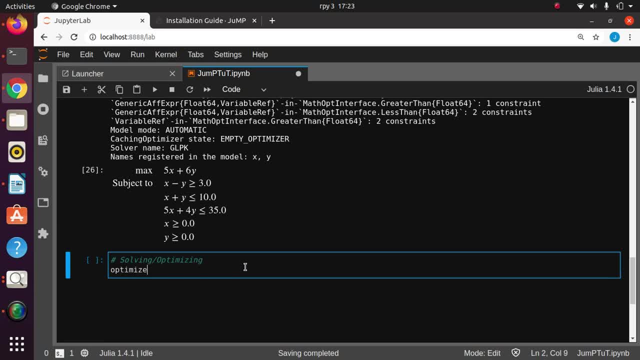 just go with my optimize, so this is a rotating function. then i'm passing my model, so this is going to optimize it and give us a result very fast, perfect. so we have seen it. we have to get our status right so we can just go with my termination status. so this one help us to know whether our model that 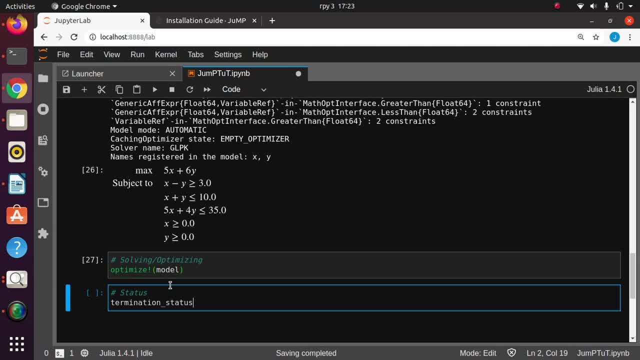 we are trying to optimize was able to arrive as an optimal solution or not optimal solution, so i'm just passing my model. so this is going to tell me that we got one. so the termination status code is one that means that we've got an optimal solution to get all of the various status codes. 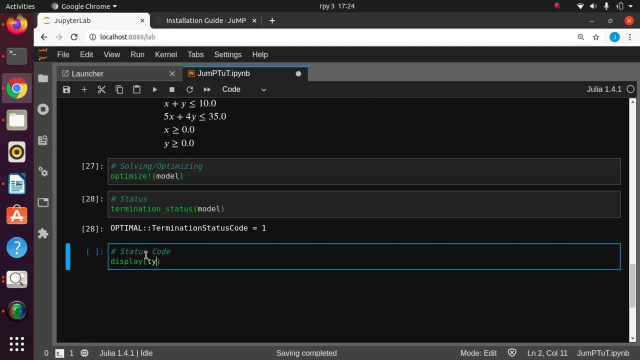 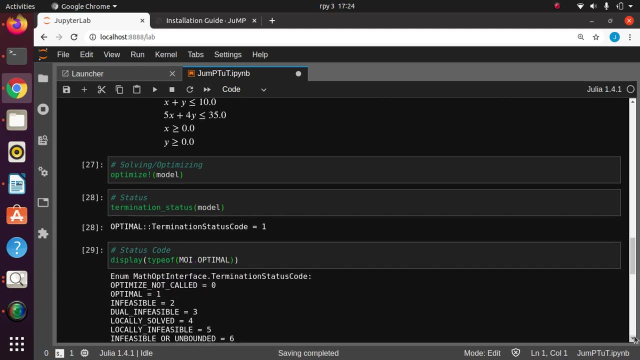 just go with my display type of: then moi dot optimize up to optimal right. so this is going to display all the various status code for determination. so these are going to be the status code. so one means it's optimal. you'll be able to find an optimal solution. 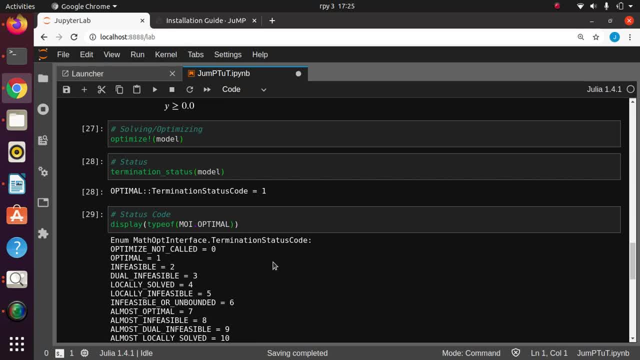 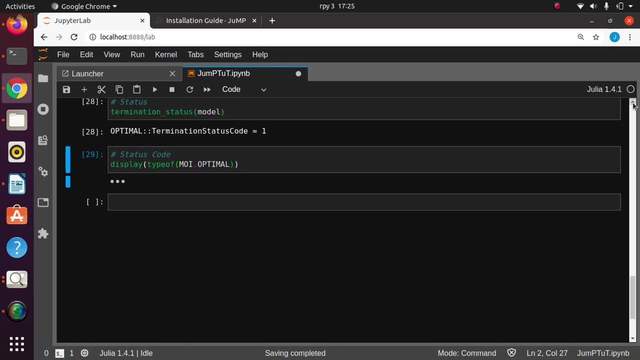 two means it's infeasible. right, that means the problem is not visible. you can't do it right in real life. very simple. so these are all the codes. now let's see how to get our actual value right. yeah, i've seen that we have gotten an optimal solution now to be able to get the values. 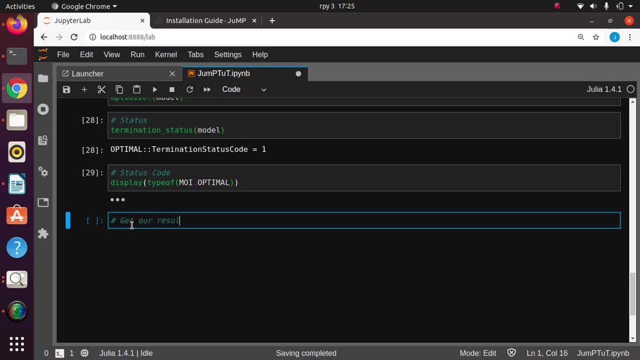 to get our result show好的. its a sure macro right. then just pass in value. i want to get my one for x show value for y, so this will give us the right values of our" that we need. so these are the values that we need. so we need five of x and two of y to be able to. 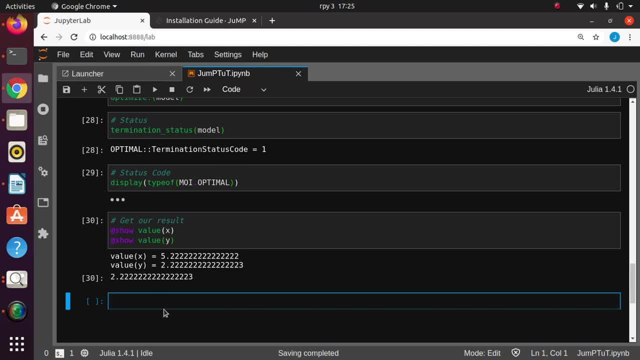 give us our maximum result for that particular function. so let's check for the objective value. so to get the objective value, just go with this, the objective value. so you can just go with this show objective value and i'm passing my model so this is going to put in this particular 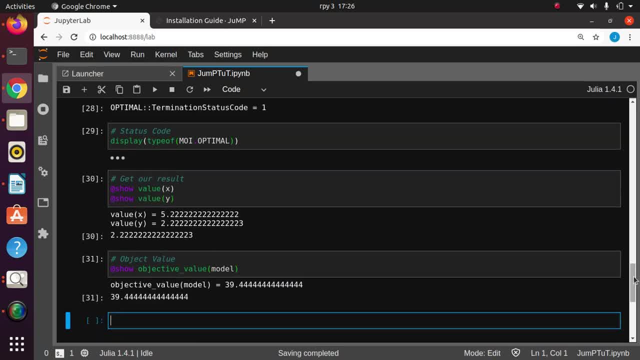 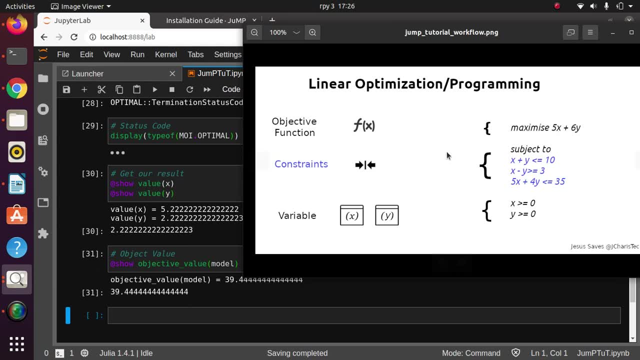 value that we have into our optimization function and return our result. very simple, right? so that is something very simple. so i've seen how to do simple linear programming using jump by defining our variables, constraints and an objective function. so it's something very simple. so if i put in these values- f and x, right x and y- into my objective function, if i put it back into 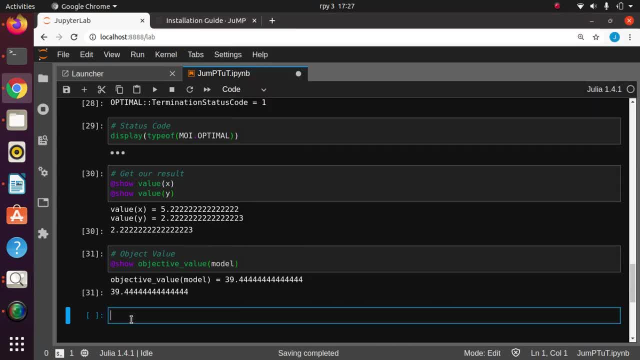 my objective function, i'm going to get the right result. so let's try an example. so we realized that our objective function was f. s plus says y, right, so if i put in these values, i might get this. so let's try it. it's going to be this: